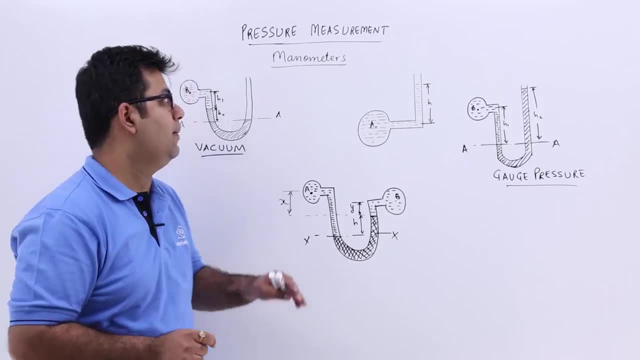 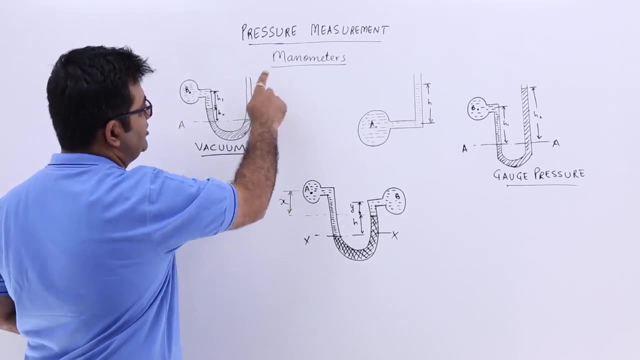 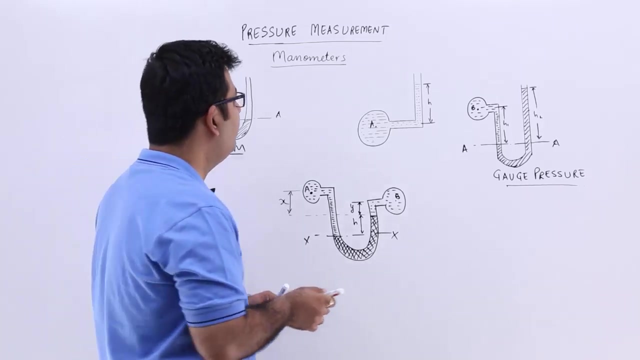 Now, after Pascal's law, let's talk about manometers, which is a pressure measurement device. How does this device measure pressure? The pressure is measured by a manometer by balancing this pressure against a column of liquid, And that column of liquid is in static equilibrium. 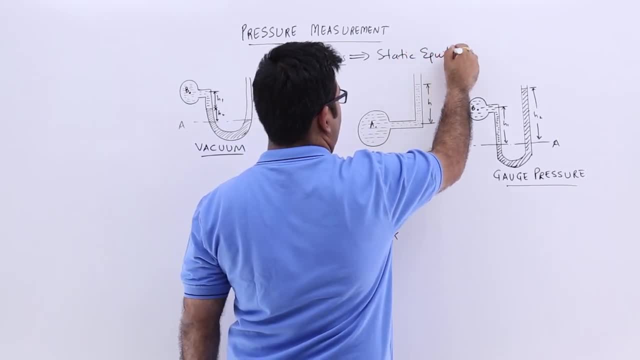 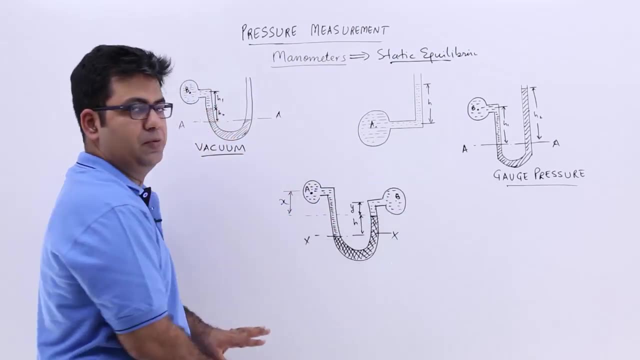 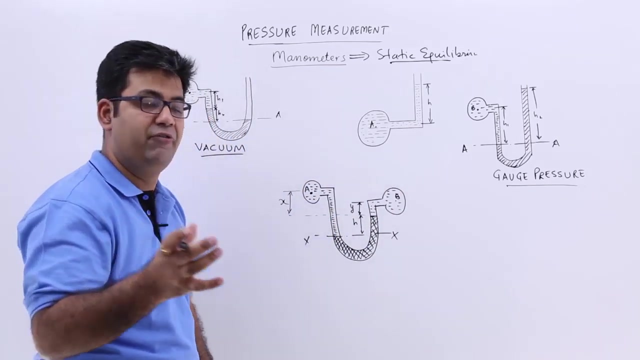 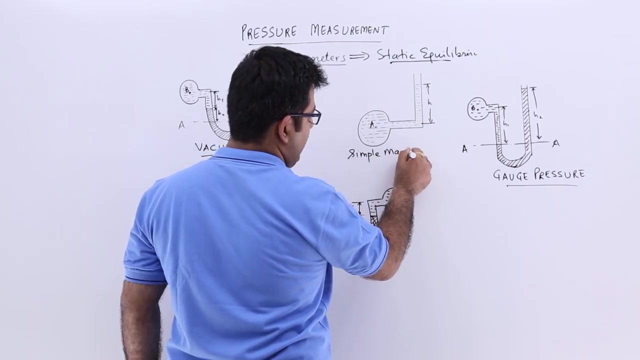 So this word is very, very important. Okay, so if you look at this figure, first of all forget all the figures on the board, just focus on this figure. This is how a manometer looks like. So this is the simplest form of the manometer, which is called a simple manometer. 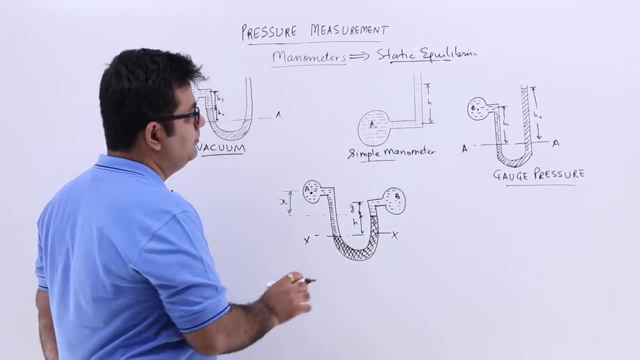 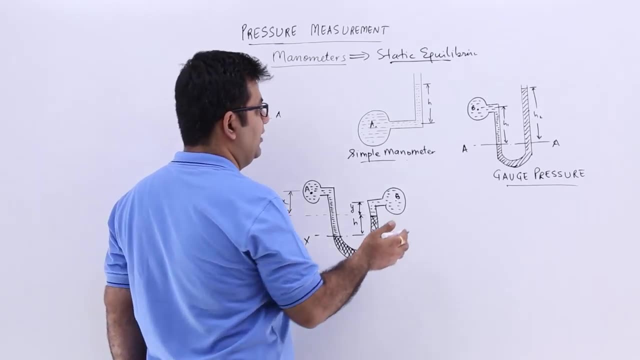 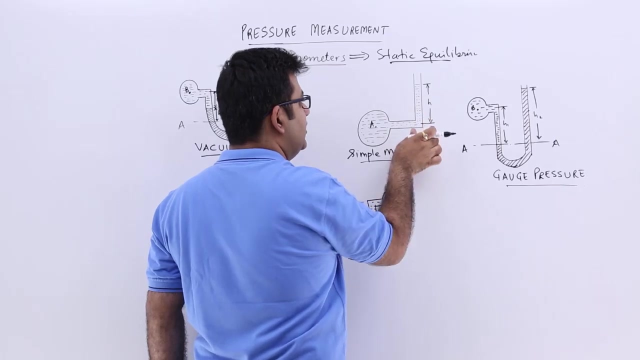 Okay, so what is happening in this device is you have a certain vessel, In vessel which we have some fluid or a liquid, Okay, And we have to measure the pressure of this liquid inside this vessel. Now, this vessel is connected to a vertical tube. 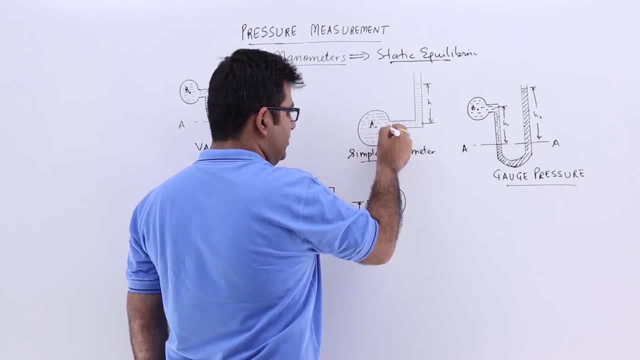 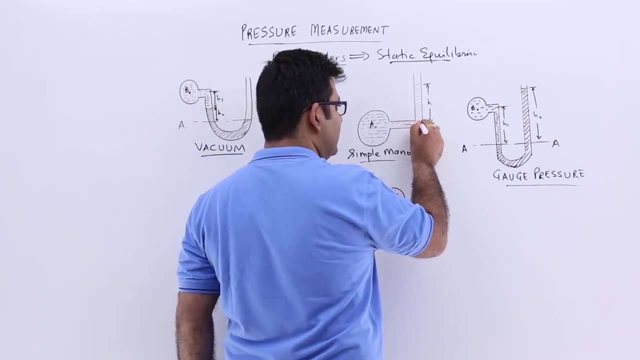 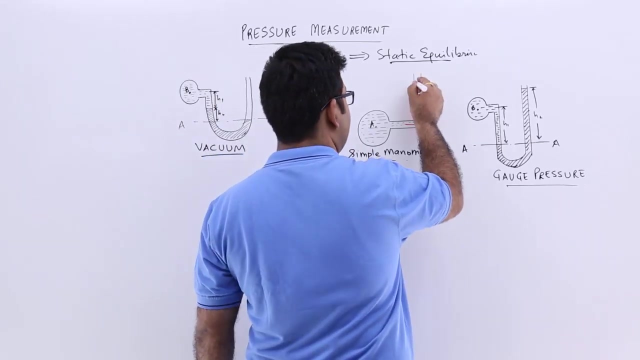 So what happens is that, whatever the pressure is inside this vessel, due to that pressure the liquid rises up in this vertical tube And it rises up to a certain height. That height is this: h. This is the height which is attained by this liquid. 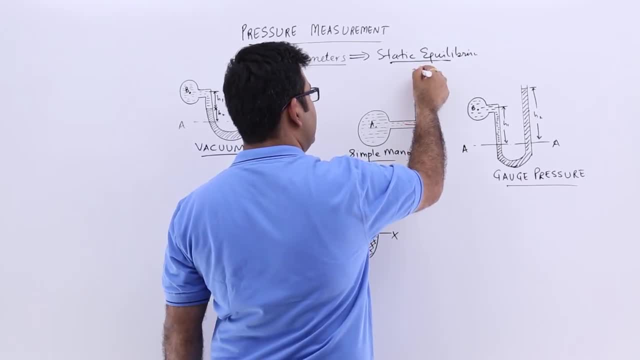 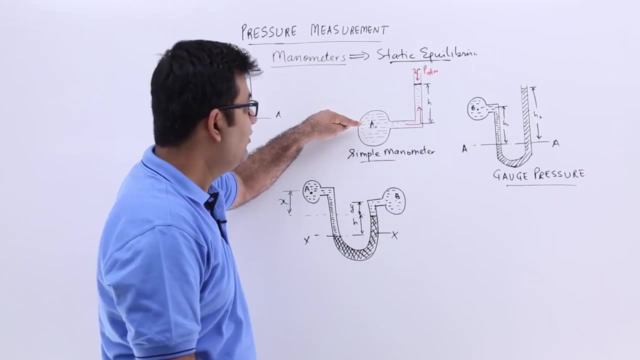 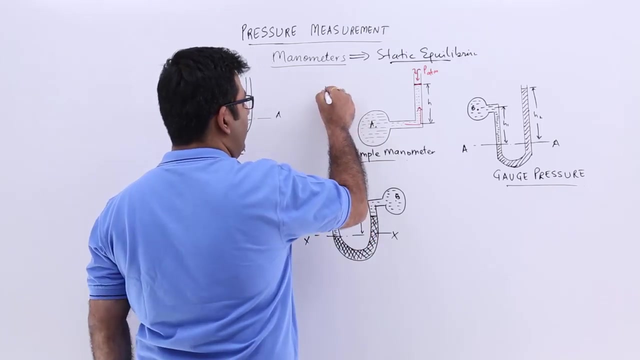 And it balances the atmospheric pressure on top. Okay, So the pressure inside this vessel is equal to the pressure of the liquid column which is at a height h. So to find out the pressure at point a, this is equal to rho, which is the density of this liquid. 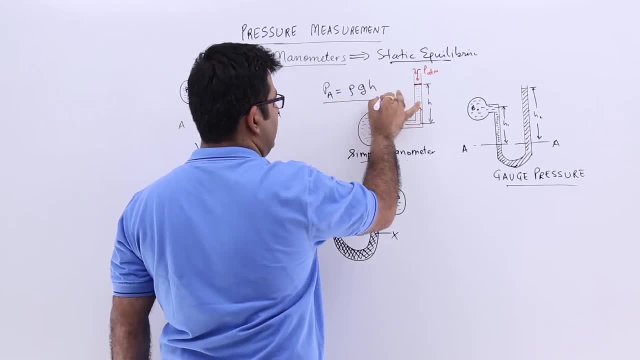 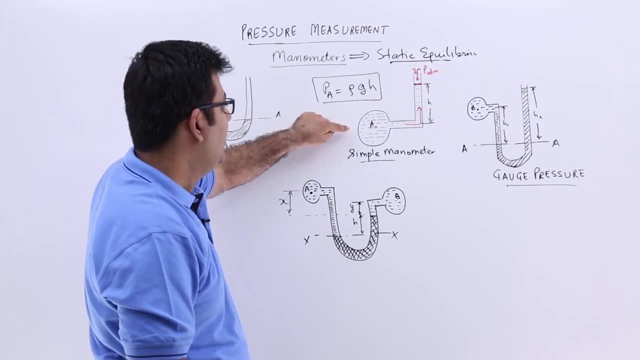 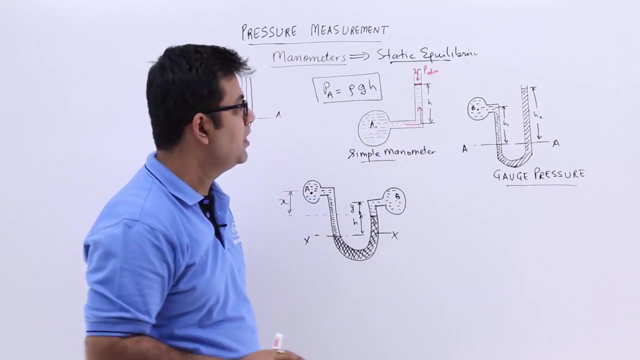 Into g, into height. So that is the mathematical formula to find out the pressure in this vessel with the help of a simple manometer. Okay Now, this is a very simplistic arrangement. You can also use a u-tube gauge. 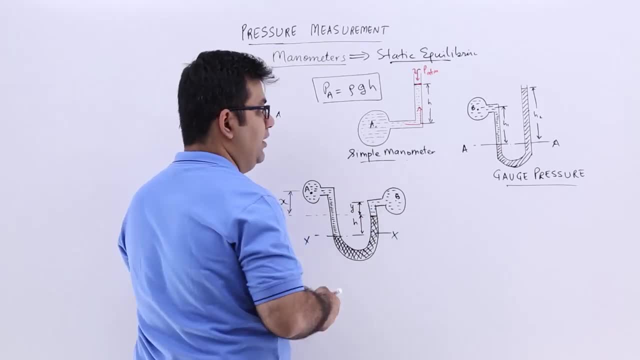 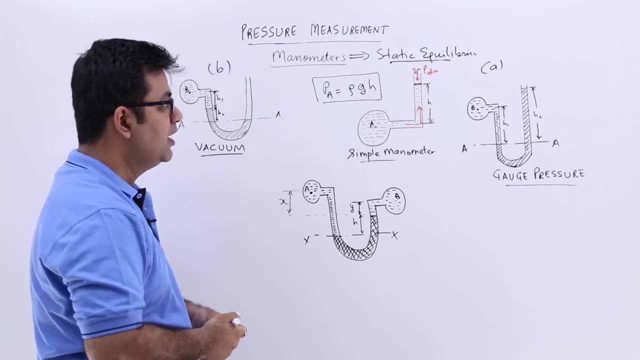 So there are two u-tube gauges, One this. So let me name this figure as figure a And this as figure b. So figure a is the arrangement In which you have two kinds of liquids. In the simple one, you just have one liquid. 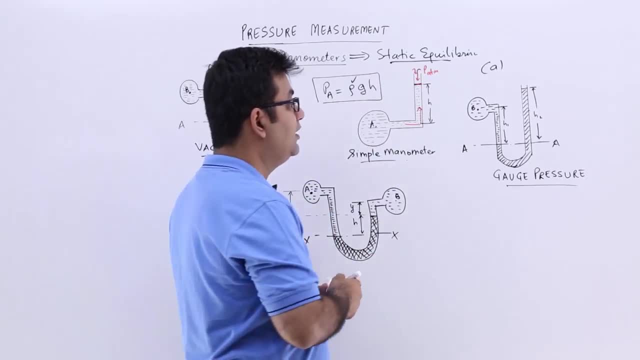 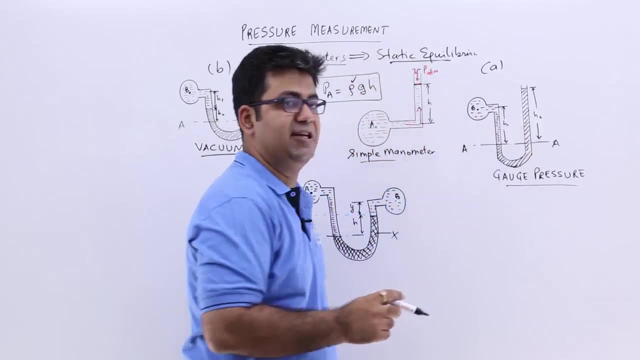 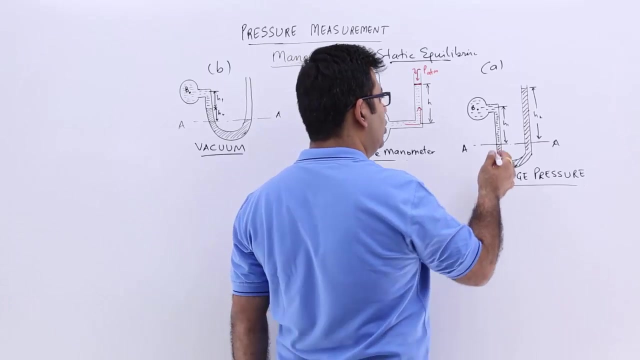 So you just have one density to take care of. But in this a and b you have two liquids, Okay. One is the liquid for which the pressure has to be measured And the other one is a heavier liquid. Okay, So this: 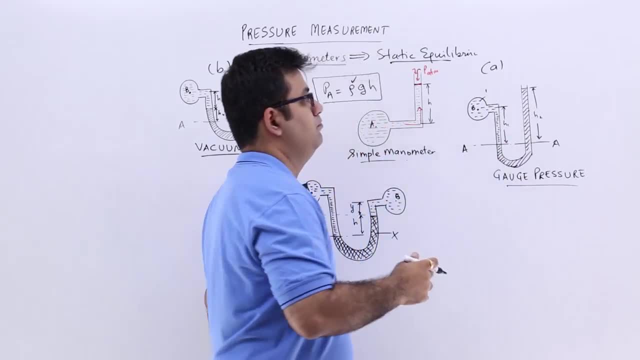 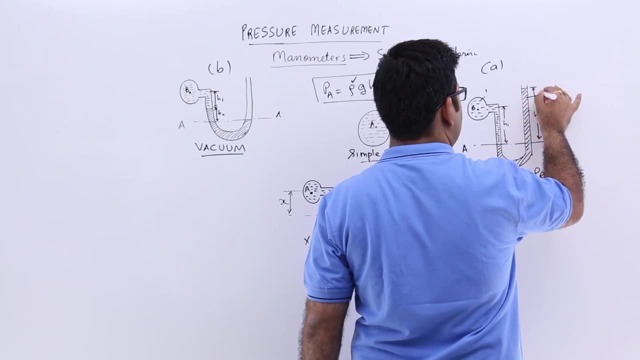 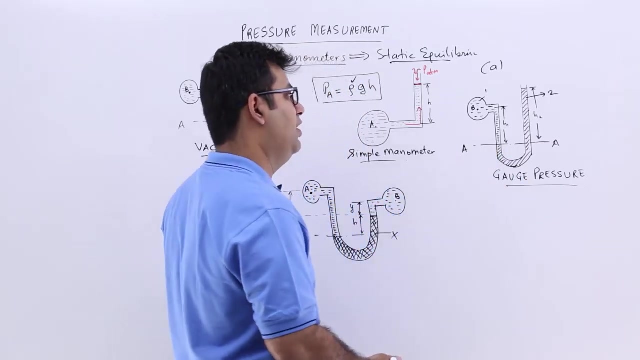 let us say is liquid one More. you know, frequently it is always water. And let us say this liquid is liquid two, which is more or less mercury, Okay, Or you can say heavier liquid. So in this what happens is: 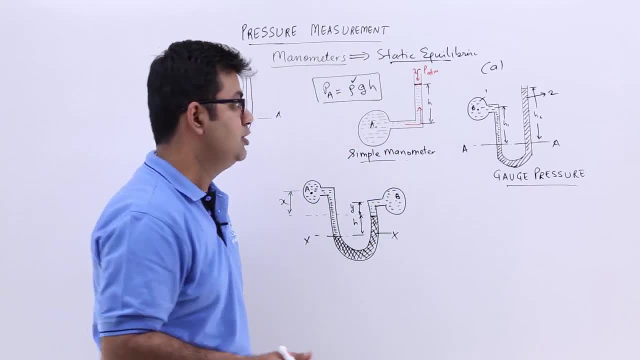 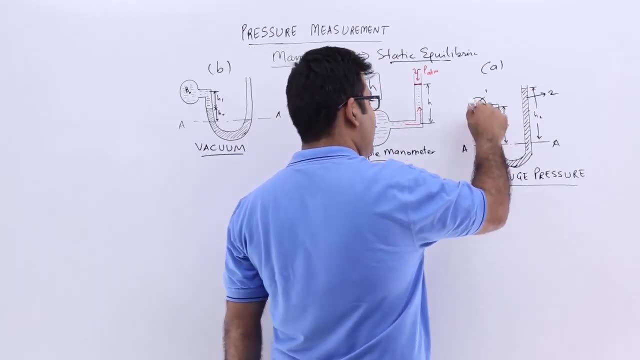 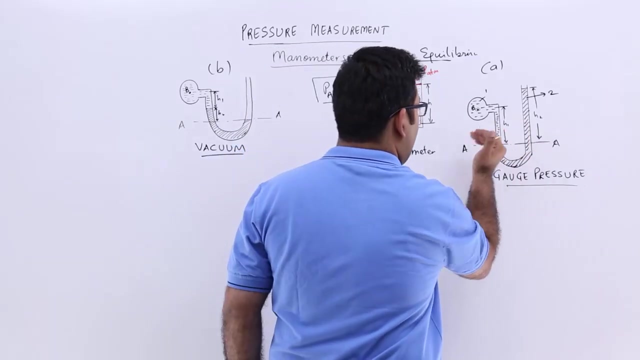 this arrangement is used to measure the gauge pressure. So the gauge pressure at point b can be measured with the help of this arrangement. So what happens is the- you can say the pressure exerted by this liquid one in the left column. 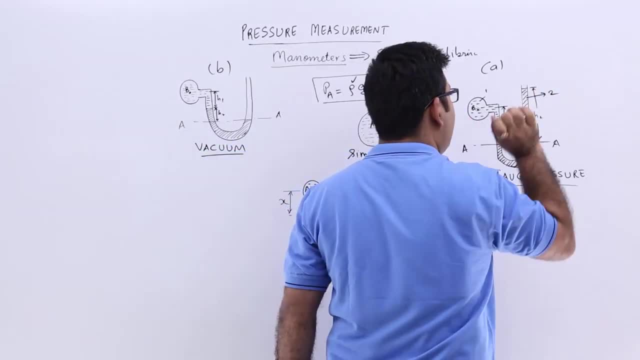 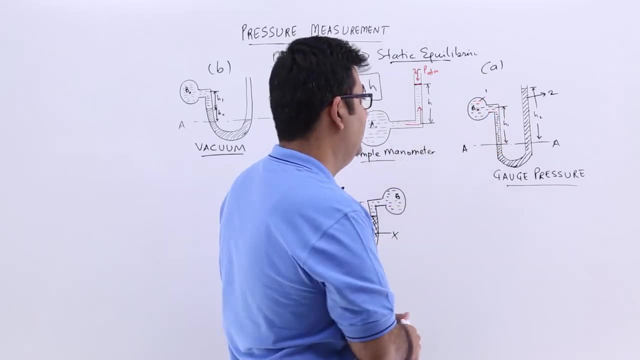 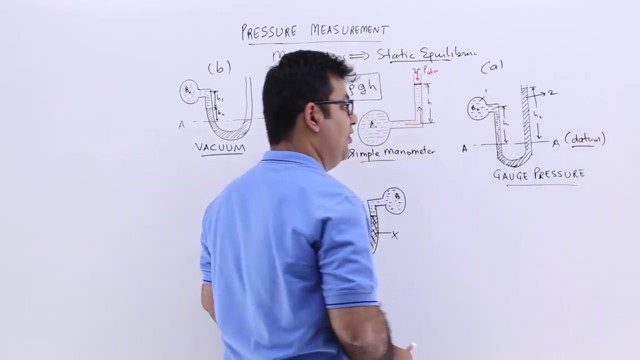 should balance in static equilibrium the height of the liquid column of the other liquid in the right limb or the right column, And this entire static equilibrium has to be, you know, calculated in reference to a datum. So we need to have a reference line. 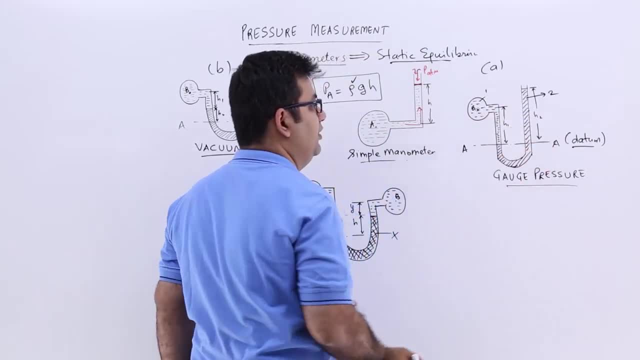 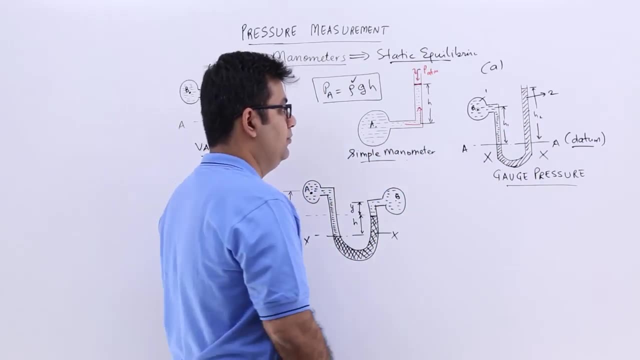 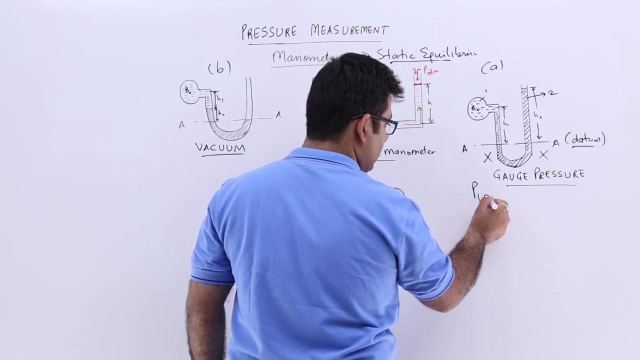 and we are doing all the calculations about this reference line, So we are not concerned with the pressure below this datum. Okay, So let us find out the pressure in the left limb. So pressure in the left limb- left limb. 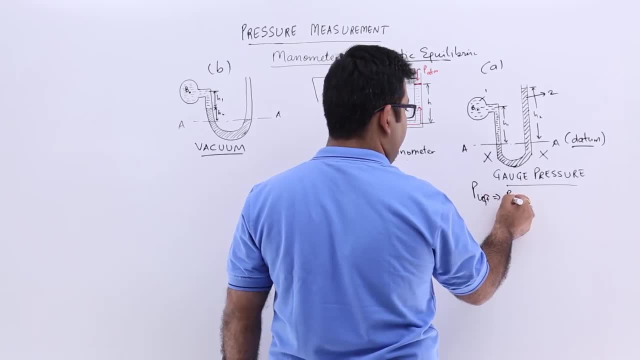 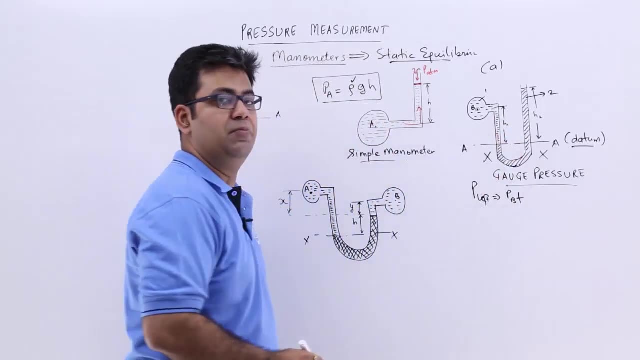 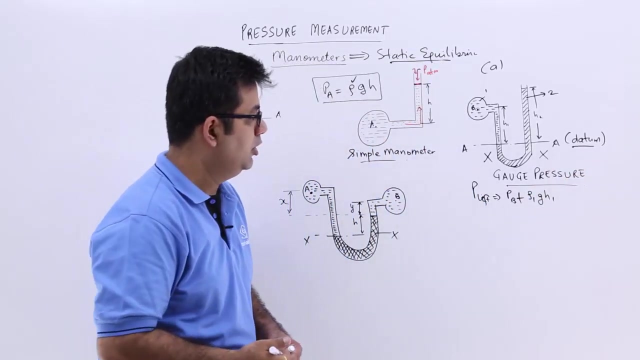 this is equal to pressure at this point, which is pressure b, Okay, This plus the pressure due to the vertical column of liquid one, So that will be rho one into g, into h one. Okay, So this is the gauge pressure. 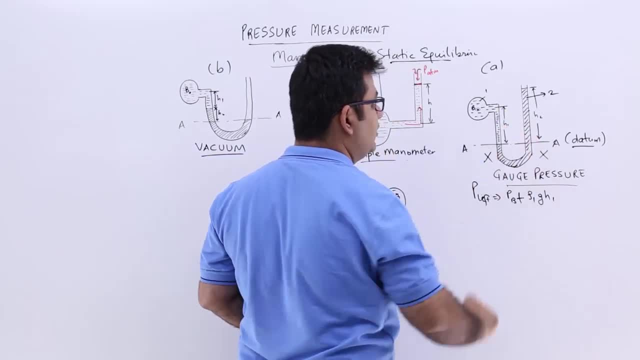 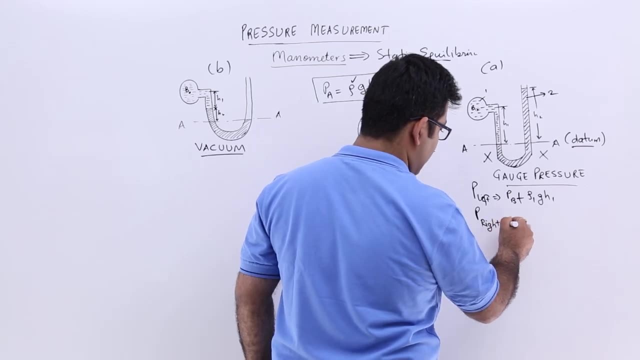 and this is the pressure on this datum due to this liquid column height. Let us find out the pressure in the right limb. The pressure in the right limb would be the pressure at this datum due to this liquid column height of. 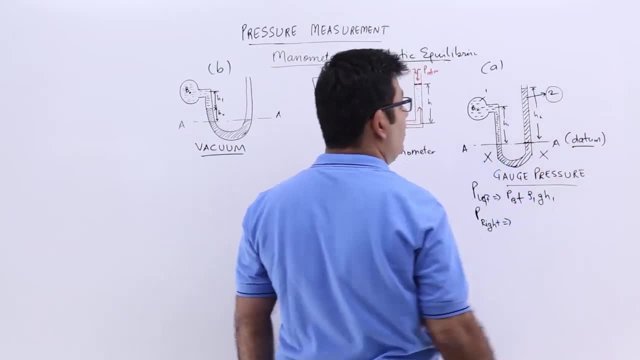 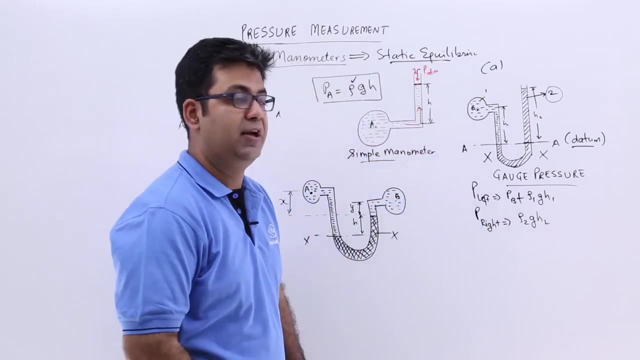 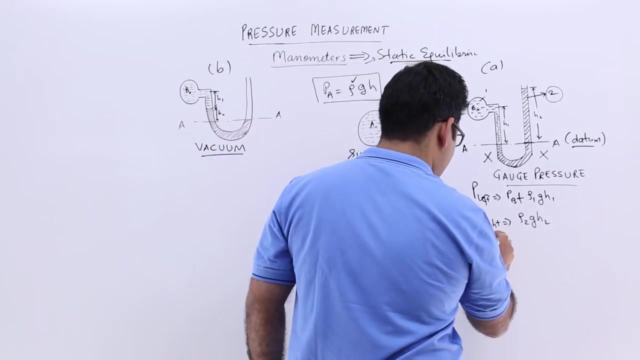 h two, which is the height of liquid of density, rho two. So you will have rho two g into h two. Now for static equilibrium. these two pressures have to equate, So you will get p b. 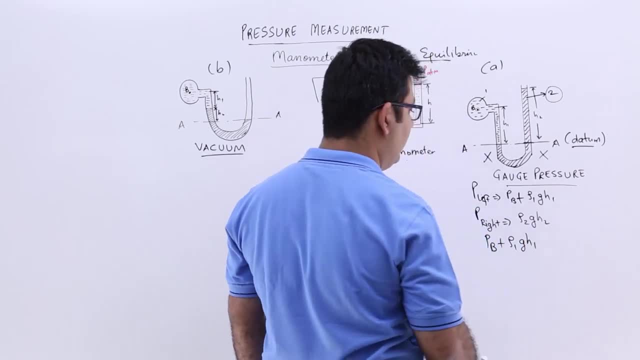 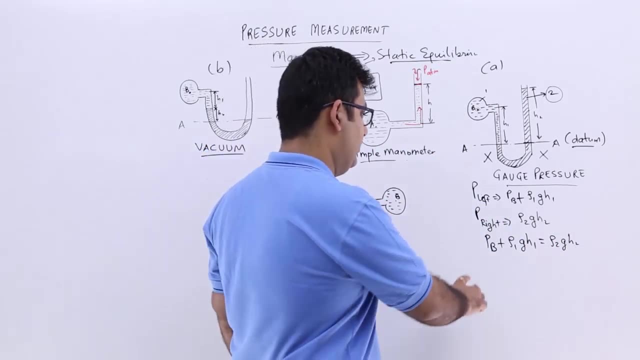 plus rho one into g one, g into h one is equal to rho two, g into h two. So from this I can find out p b. p b would be equal to rho two, g, h two. 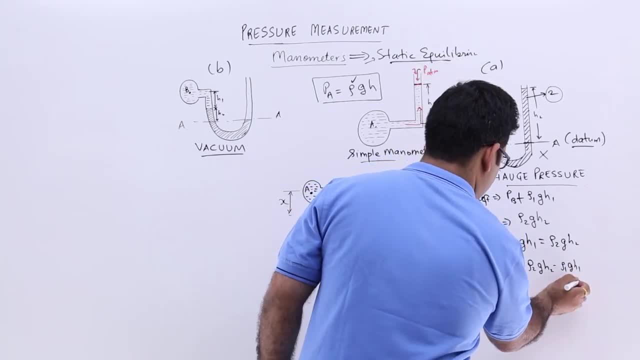 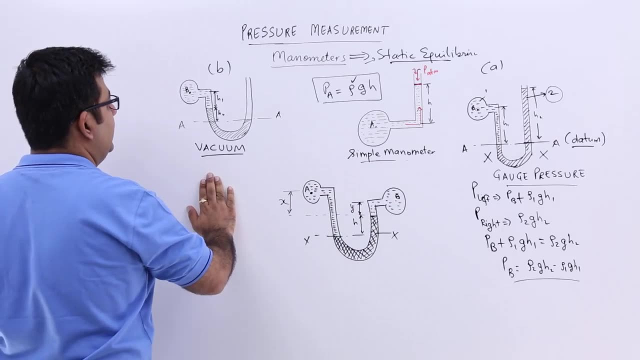 minus rho one, g, h one. So this is how you can find out the gauge pressure for this liquid. Now, if you come to figure b, that you know shows the arrangement to find out vacuum pressure. 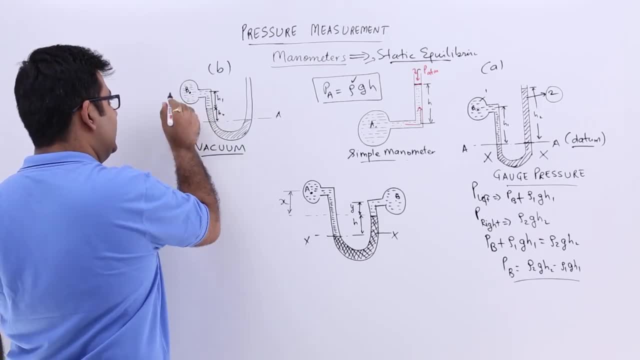 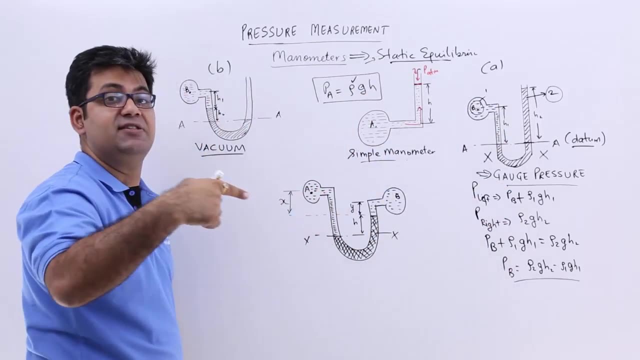 Okay, so you can see that this pressure is less Okay. so in in this, if you are finding out gauge pressure, this pressure would be higher as compared to the pressure over here. So what happens is: 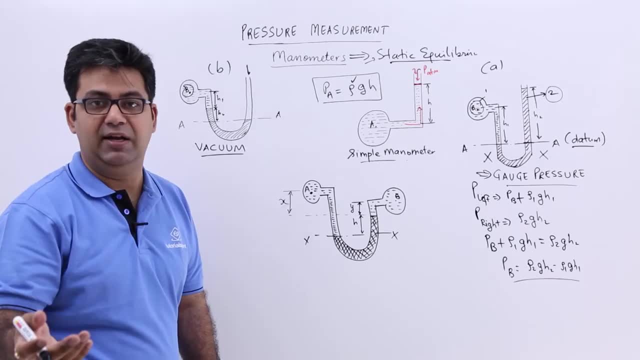 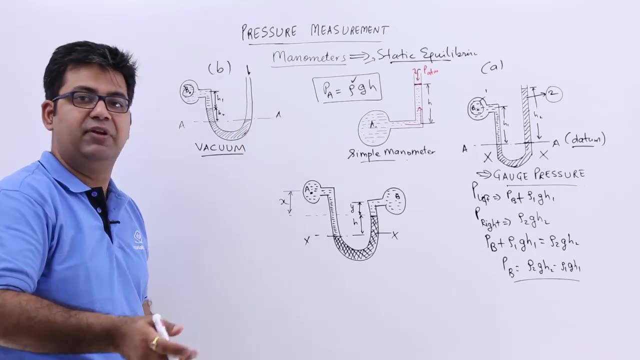 this atmospheric pressure is much larger, So this will push this heavier liquid towards the left limb. So you can see that there is no height above the datum in the, you know, in the right limb of this. 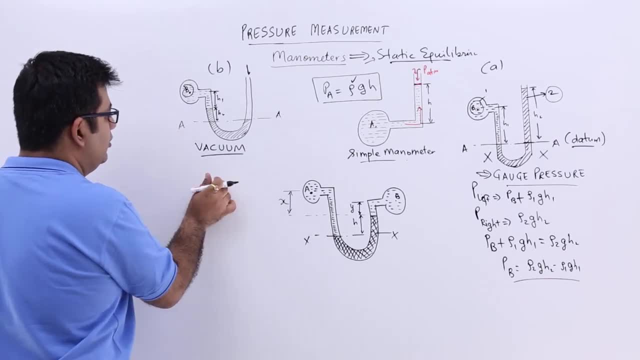 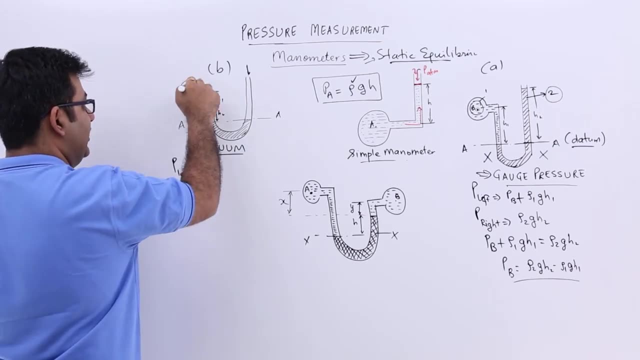 arrangement. So you will find out the p left pressure as p b, that's the pressure inside this, you know vessel, plus the liquid height, h one, So that is rho two g, h two. 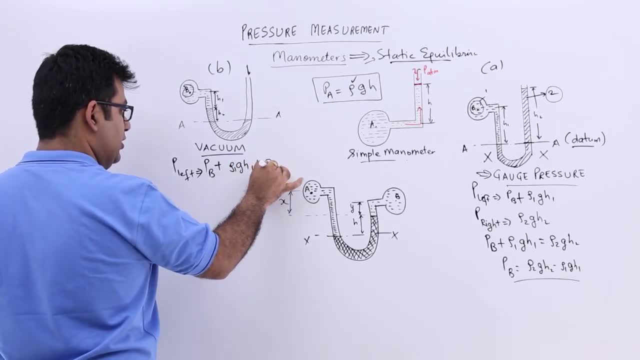 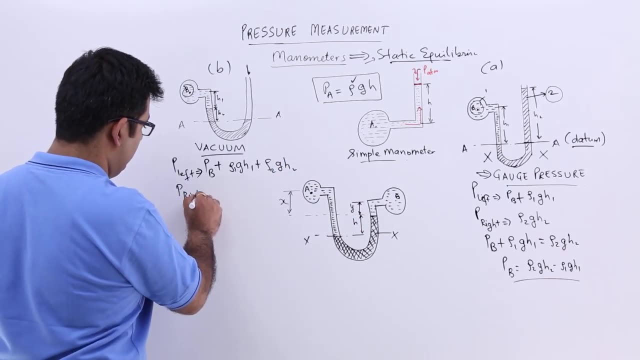 h one. so that is rho g- h one plus rho two- g- h two. And the pressure in the right limb above the datum is zero. So just equate these two pressures so you will get. 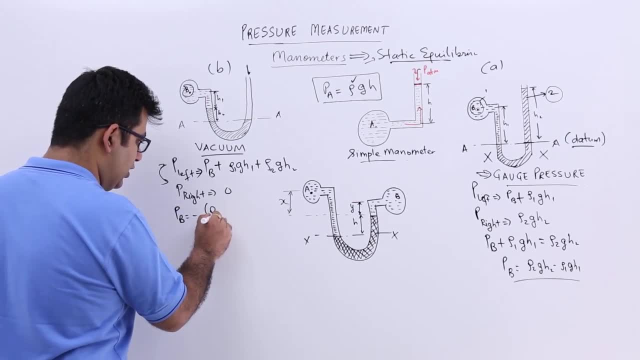 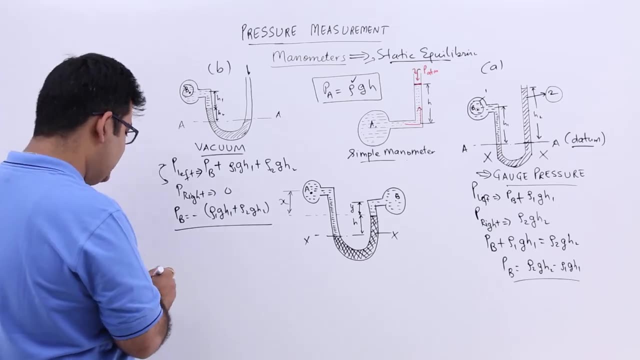 p b is equal to minus rho one g h one plus rho two g h two. So you can very clearly see that this pressure that you are getting is a negative pressure, which is for vacuum. 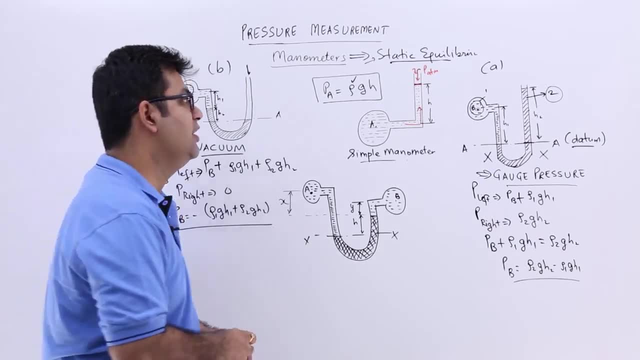 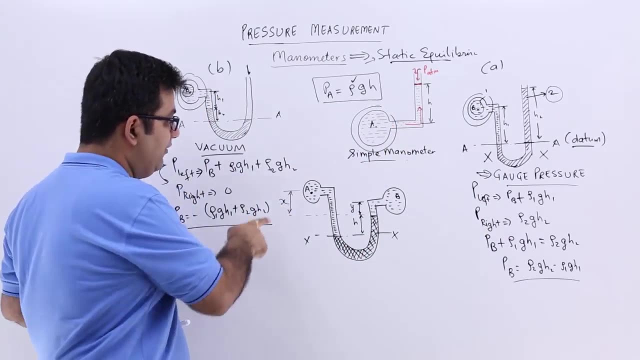 Okay, So this is how you have to calculate the pressure inside this vessel. Okay, Now, this is for a single vessel. We can also have two vessels attached with the help of a u tube, So this is called. 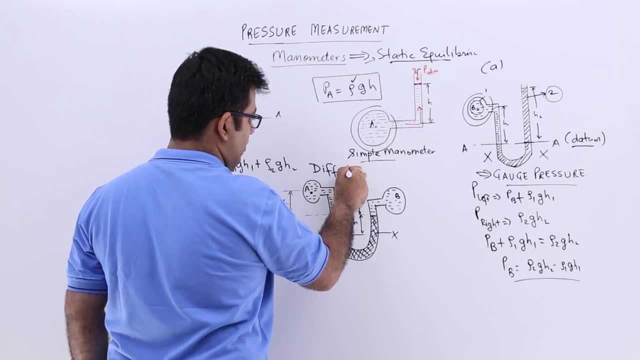 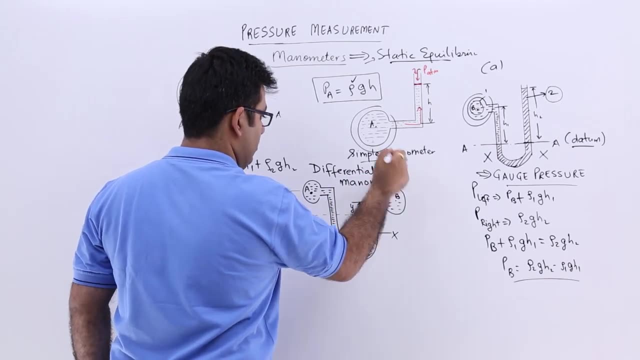 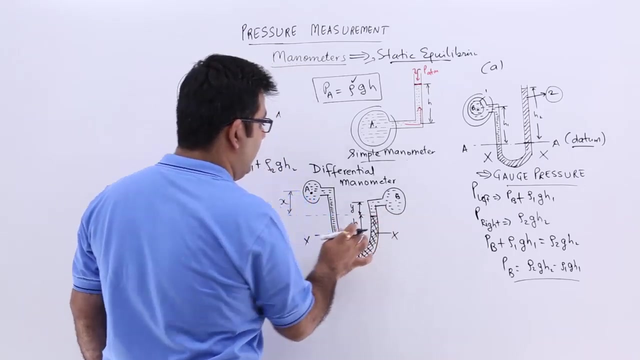 a differential manometer. Differential manometer. Okay, So what do we do with this? We do not measure the absolute pressures at a and b, but we are more interested to find out the difference of pressure. 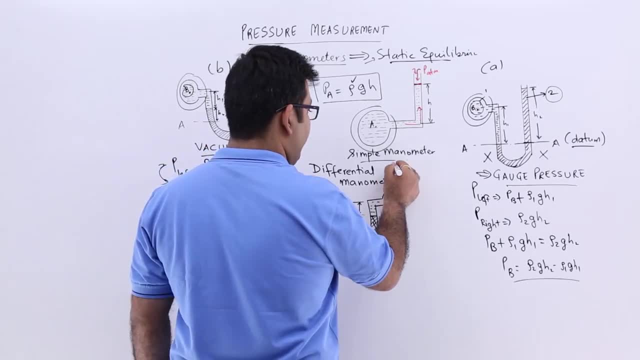 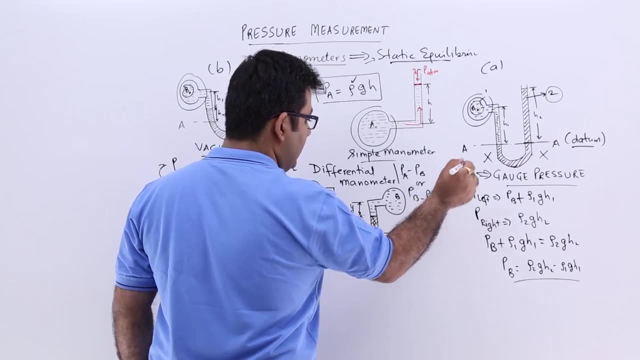 in these two vessels. Okay. So means we will be finding out either p a minus p b or we will be finding out p b minus p a, Okay. So if you look at this, it has. 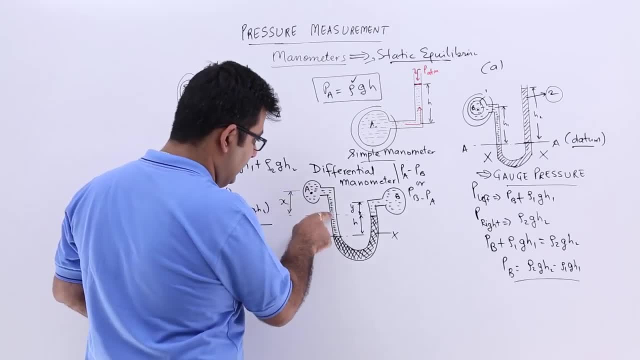 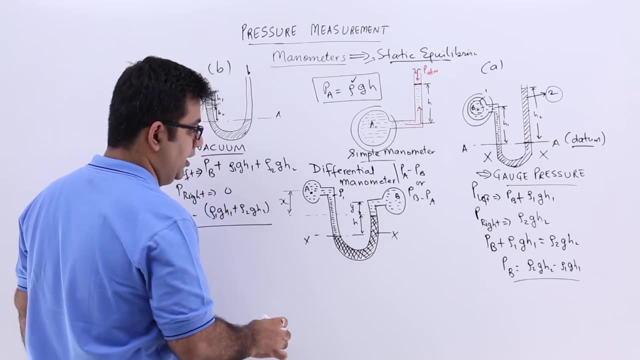 you know three liquids. So you have a liquid in the left left limb or the left column. Let us say the density is rho. 1. You have a heavier liquid. Let us say it is mercury. 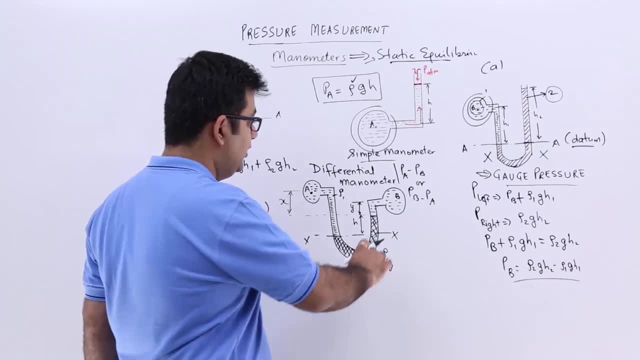 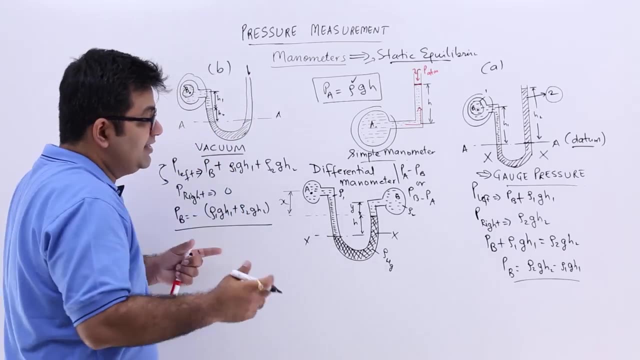 Okay, And then you have a liquid in the right limb, which is the pressure vessel b. Let us say the density is rho 2.. Now, in many cases both will have the same liquid, So you can. 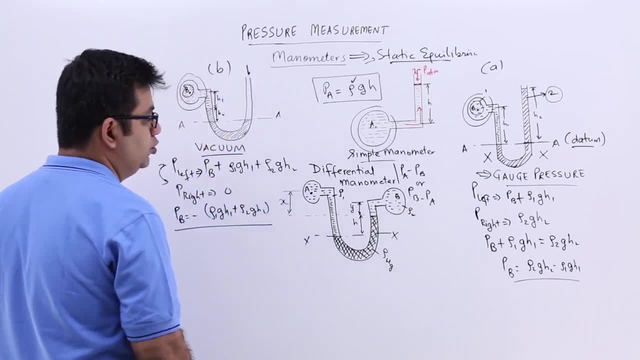 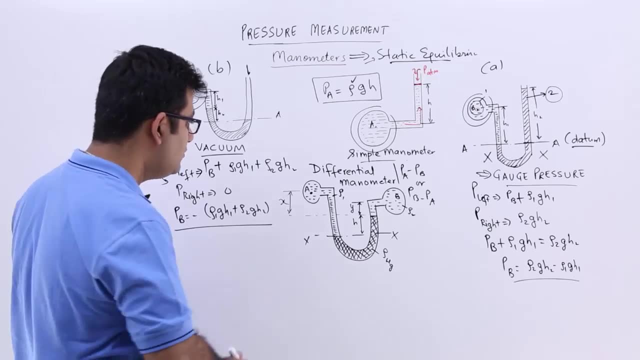 assume that the these two densities would be same, Something that is, find out the pressures in the left limb and the right limb of the atom. So let us find out for the left limb, So you will have. 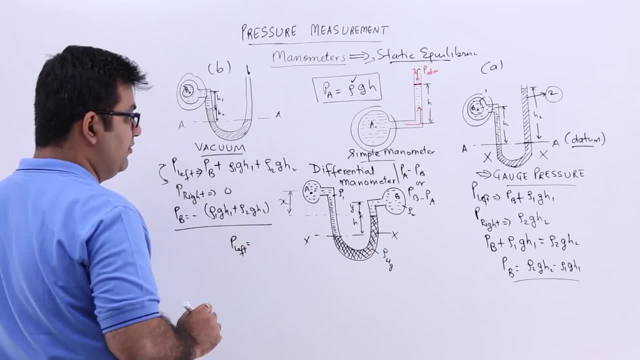 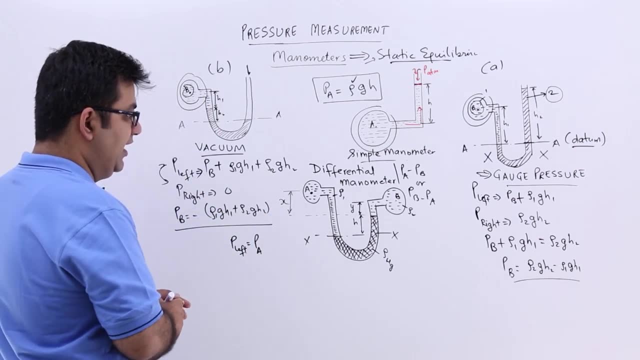 p left is equal to, you will have pressure at a Alright Plus you will have the entire liquid column for density, rho 1.. That is rho 1 g into h plus x. 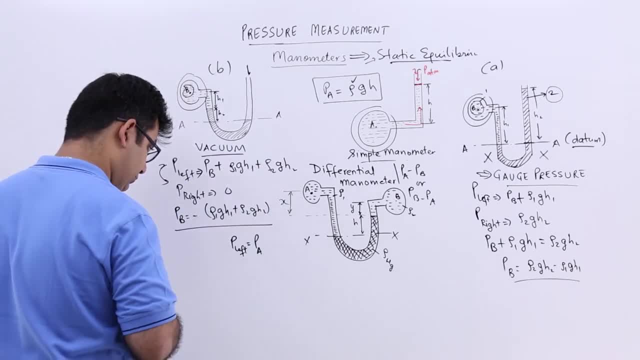 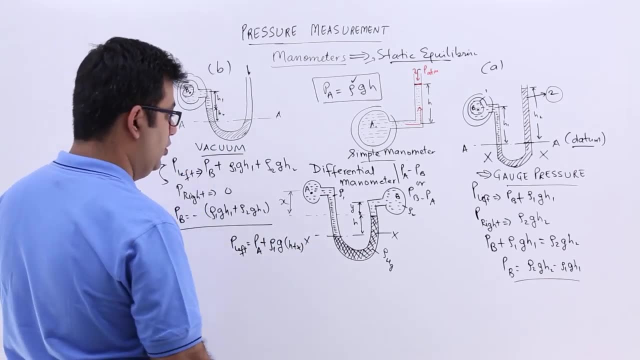 Okay. So rho 1, g into h plus x. Okay, That is for the left hand column. Now let us go to the right limb or the right column, So you will have p right. 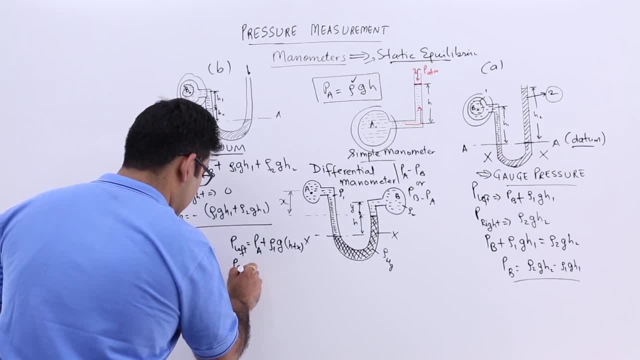 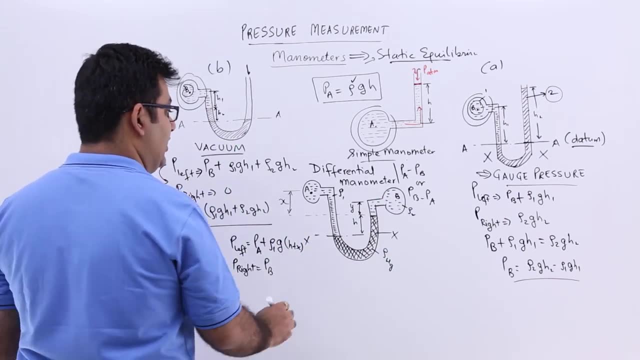 This is equal to. so you have that pressure p b. Okay, And then you have the liquid column of rho 2, for height y. So this will be plus h plus x. This will be.